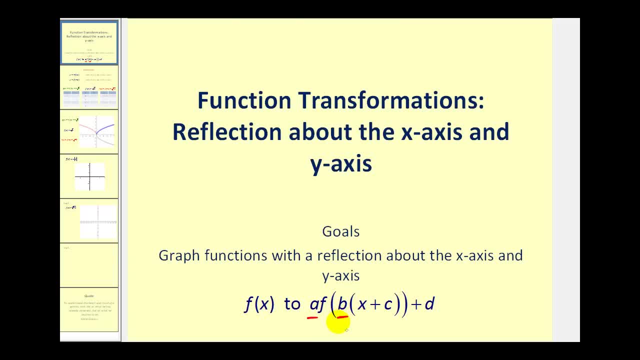 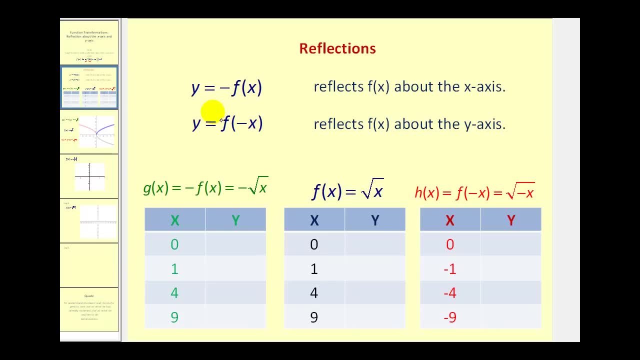 affect the graph of the original function. So, even though we have talked about vertical and horizontal stretches and compressions, we haven't talked about what happens when we change the sine of a and b. y equals negative, f of x reflects f of x. about the x-axis, Remember: f of x is equal to y. 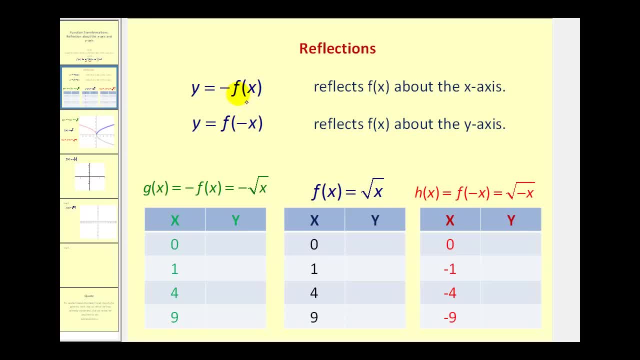 So if we change the sine of the y-coordinates, that would reflect the graph about the x-axis. If y equals f of negative x, this would reflect f of x about the y-axis. And here we're changing the sine of the x-coordinates and therefore 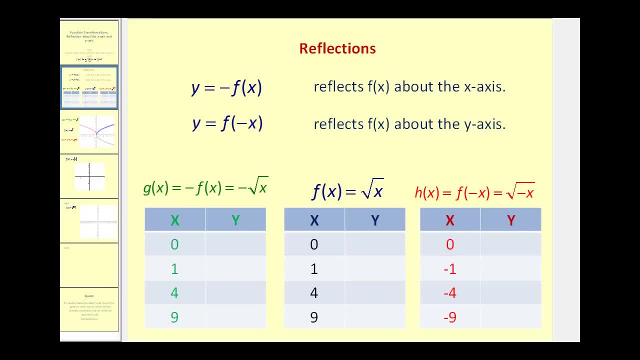 will reflect the graph across the y-axis. Let's go ahead and take a look at this using t-tables for comparison. If f of x equals the square root of x, then to determine y we would take the square root of these x values. So the square root of zero would be zero. the square root of one is one. 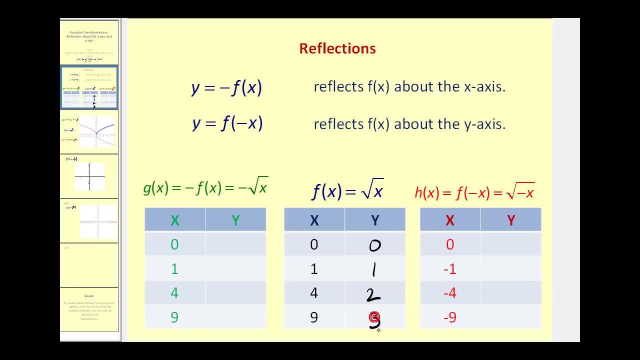 the square root of four would be two. the square root of nine would be three. Now let's compare this to g of x, which equals negative f of x, which equals negative square root x. So the square root of x would still be the. 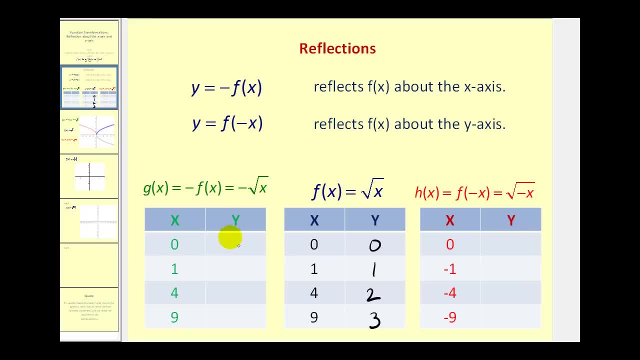 same each time. but now we would take the opposite of that, So we would have zero negative one, negative two and negative three. And notice that if you change the sine of the y-coordinates, this would reflect the graph across the x-axis. 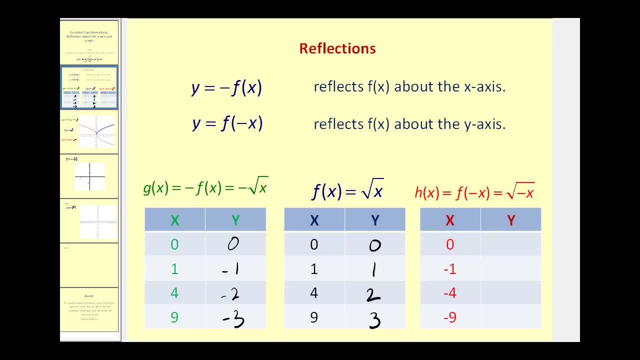 Now, if we let h of x equals f of negative x, this would equal the square root of negative x. Remember this: radicand must be greater than or equal to zero to take the square root of it. So if we change the sine of the x-coordinates, 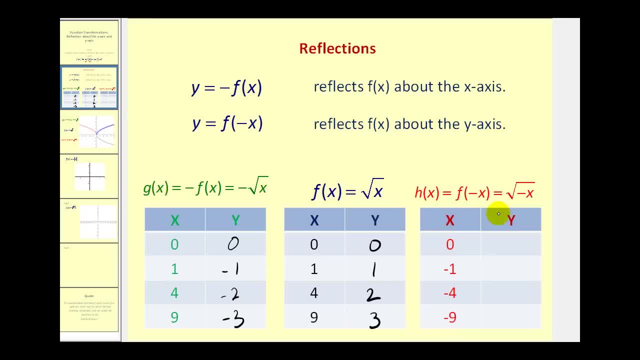 so if we change the sine of our input with x would make our radicand either positive or zero. So we'd have zero, one, two and three. So since we changed the sign of the x-coordinates, it would reflect it across the y-axis. 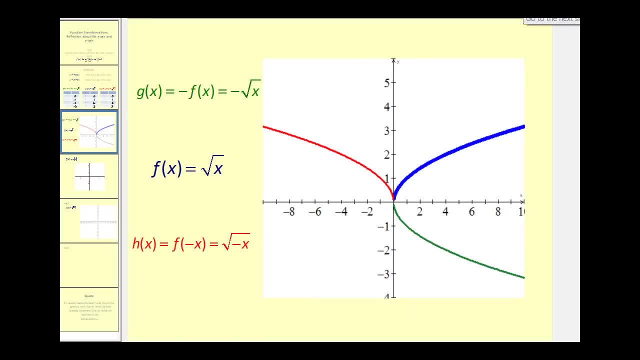 If we were to graph these three functions on the same coordinate plane, we would have our original function in blue If we change the sign of the x-coordinates. if we change the sign of the x-coordinates or reflect this graph about the y-axis. 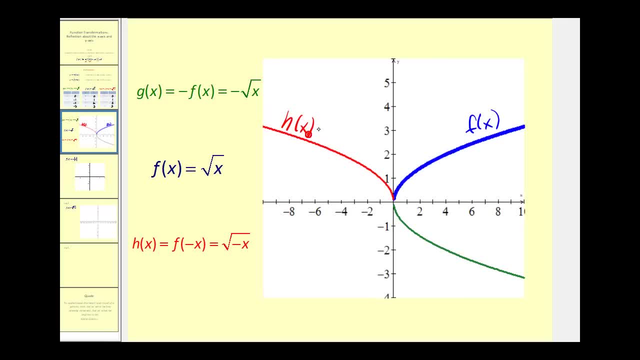 we would have h of x, which equals f of negative x. We'd change the sign of the x-coordinate And in green, if we reflected across the x-axis or changed the sign of the y-coordinates, we would have g of x, which equals negative f of x. 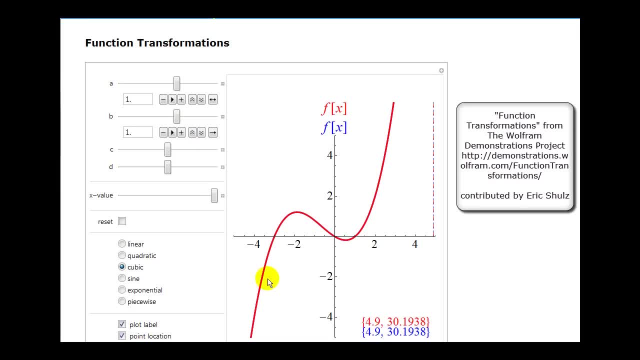 Let's take a look at an animation of this. So what we see here is the original function in red, and we'll see the transformed function in blue. We'll start by changing the value of a from positive one to negative one. Here you are seeing a vertical compression. 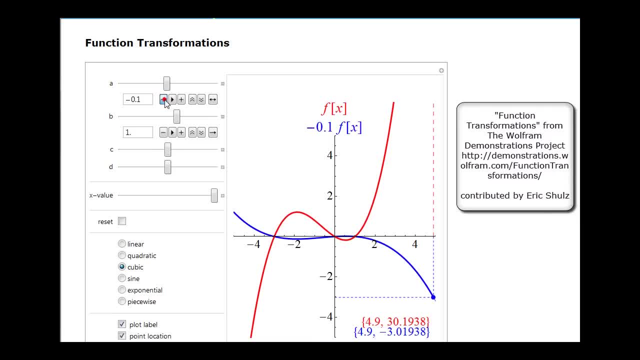 and then, as soon as a turns negative, we'll see a reflection across the x-axis, And as soon as a equals negative one, the transformed function in blue is a perfect reflection of the original function in red across the x-axis. Let's now take a look at what happens. 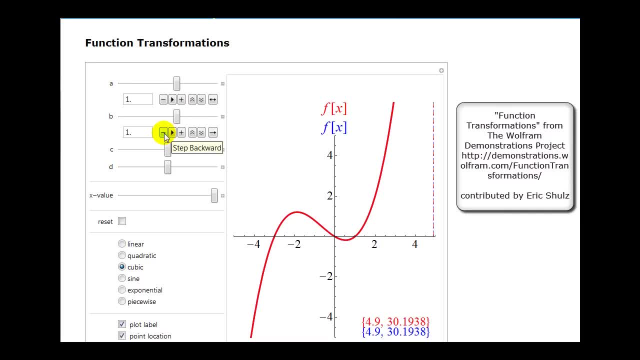 when b changes from one to negative one. So right now b is equal to positive one and as we decrease b you'll see a horizontal stretch, and then, when b turns negative, we'll see a reflection across the y-axis, And when b equals negative one, 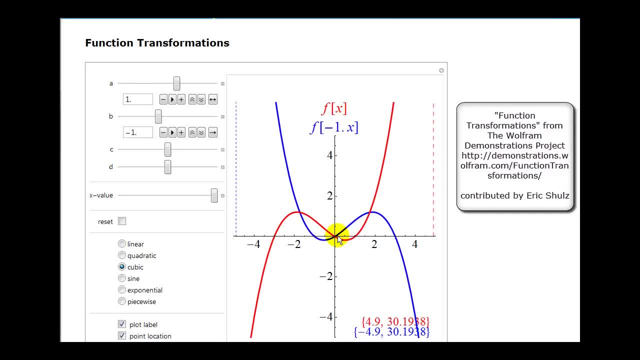 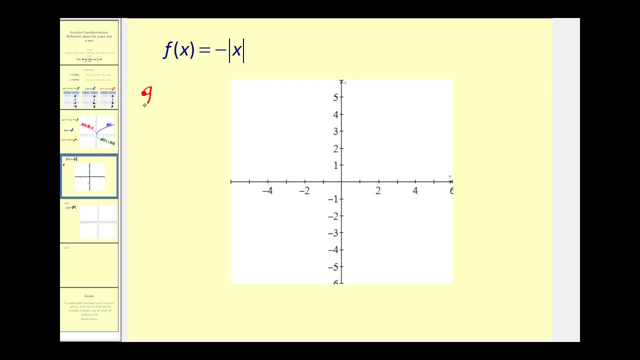 we have a perfect reflection of the red function across the y-axis. Let's go and take a look at some of our own examples now. Again, the first thing we want to be able to recognize is that our parent function, which is negative one. 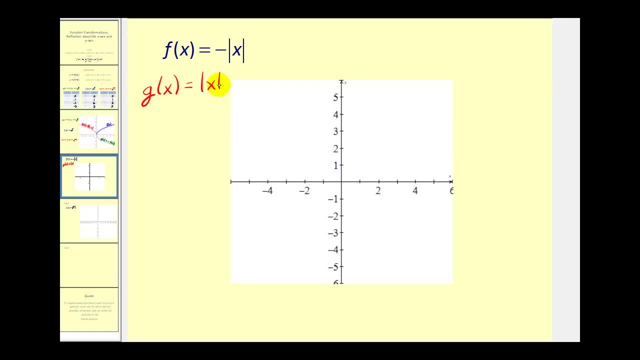 will be negative one. So we'll do that by placing the x in the vertical expression, so that it's not using the stick, and then that x in the vertical expression will be: g equals the absolute value of x, which we should know by now is just a v that opens upward. 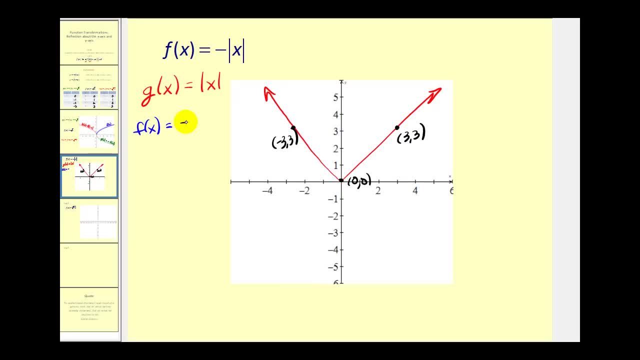 and some of the key points on this graph would be zero, zero, three, three and then maybe negative, three, three. So f is really just the opposite of g, that we're changing the sign of the y-coordinates. Therefore it's a reflection across the x-axis. 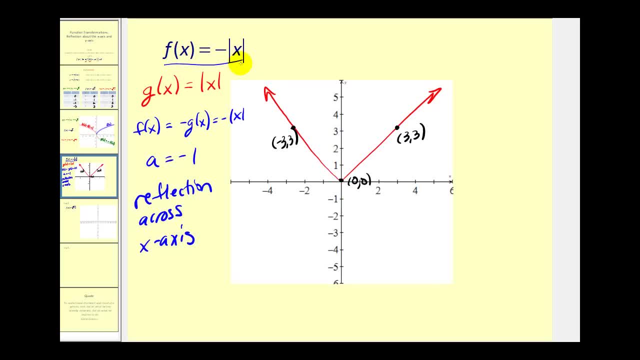 So instead of opening up, the given function will open down. So we can just change the sign of these y-coordinates. So we'd have the point: negative three, negative three, still the origin, and then three negative three. This would be the graph of f, of x. 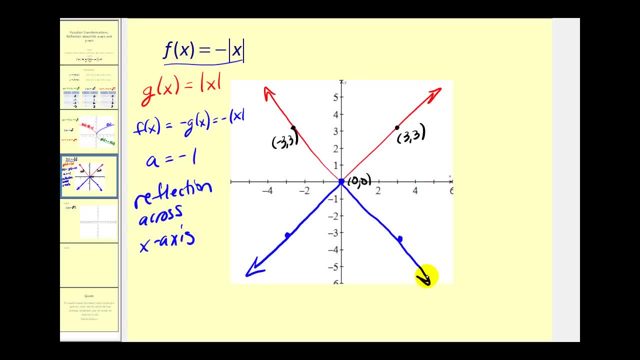 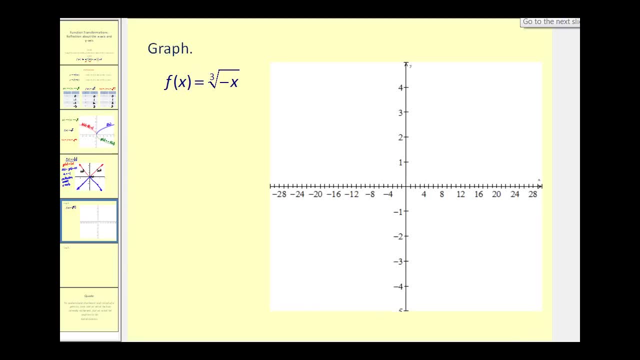 equals negative absolute value of x. Again, the original is in red and the transformed or reflected graph is in blue. And here we have: f of x equals the cube root of negative x. So our parent function would be the cube root of x. 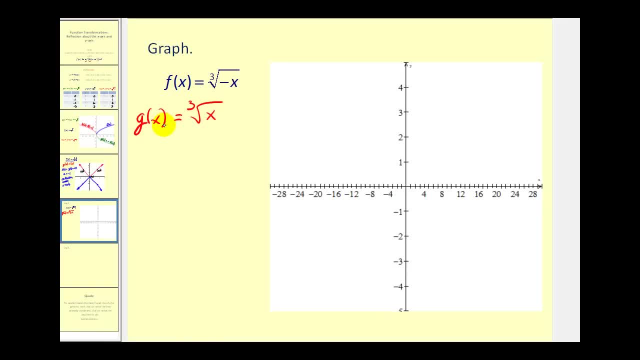 Now this one may not be quite as obvious as some of the others that we've done. Let's go ahead and sketch this parent graph. So if we take the cube root of negative eight, that would be negative two. So we'll plot the point: negative eight, negative two. 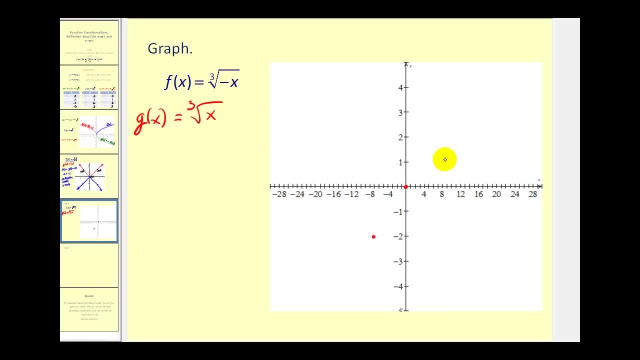 Zero, zero, And then the cube root of eight would be two. Let's find two more points. The cube root of negative 27 would be negative three somewhere here, And the cube root of positive 27 is three. So the parent function looks something like this: 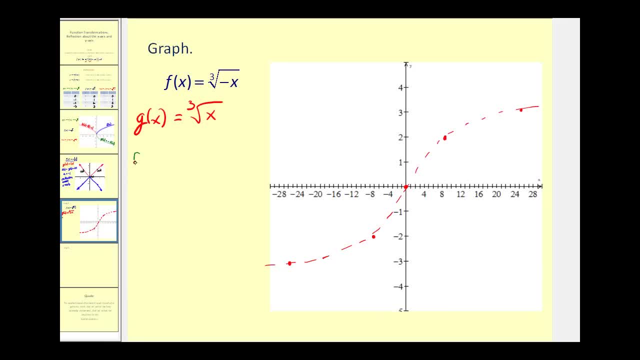 But we want to graph: f of x equals the cube root of negative x. So f of x is equal to g of negative x. So f of x is equal to g of negative x. So f of x is equal to g of negative x. 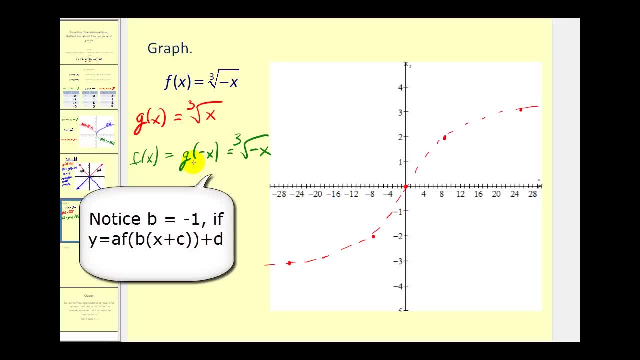 Which is equal to the cube root of negative x. So here, notice, we're changing the sign of the input or every x coordinate. So let's go ahead and just replot these points by changing the x coordinates, So we still have zero, zero. 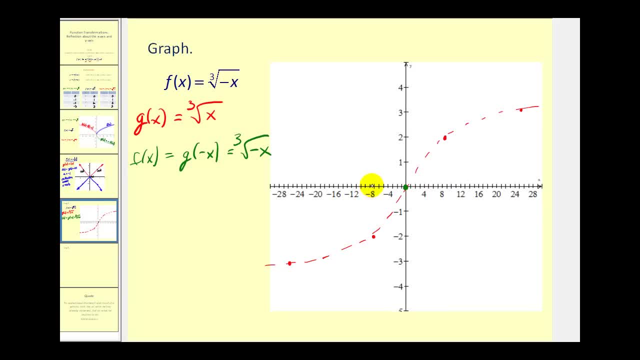 Then, instead of eight two, we'll have negative eight two. Instead of 27, three, we'll have negative 27, three. And instead of negative eight, negative two, we'll have positive eight, negative two And, lastly, instead of negative 27,, negative three. 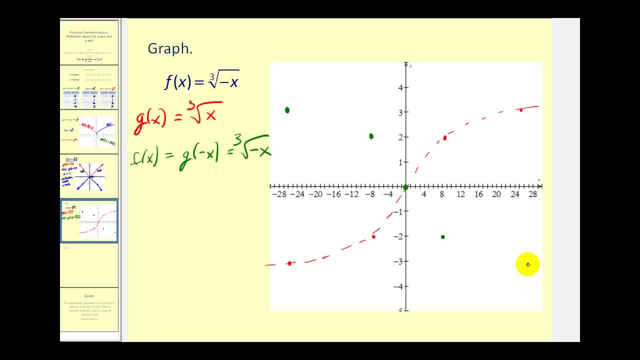 we'll have positive 27,, negative three. So our transformed graph is green and would look something like this, And now we can see it's a reflection about the y-axis. OK, In the next two videos, what we're going to do is take a look.